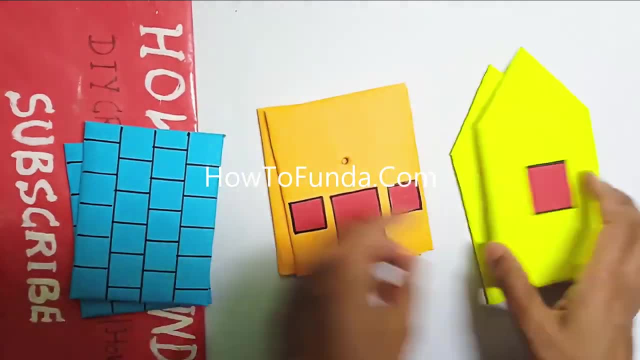 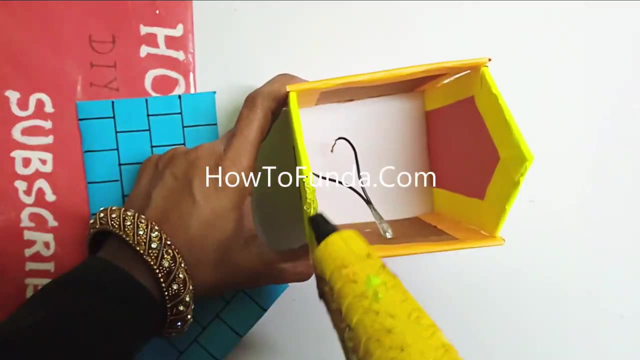 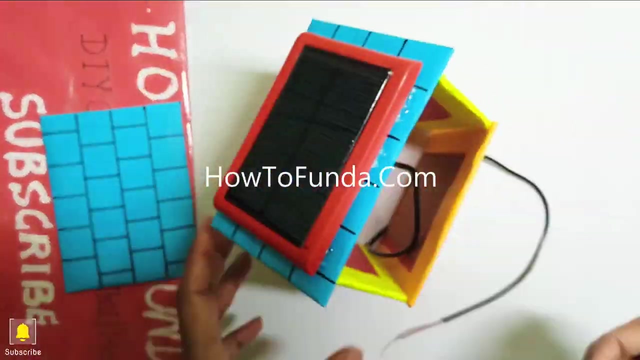 They want to rise up while you drown. They want to fill your head with doubt. They're silently scared that you'll figure it out. I'll make it look like I'm losing, Won't bother hiding my bruises. And when they finally think you're wounded, 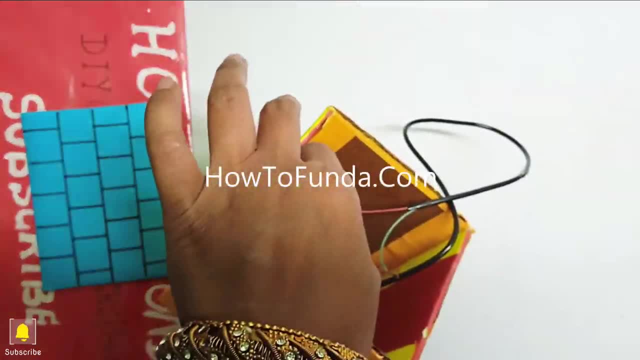 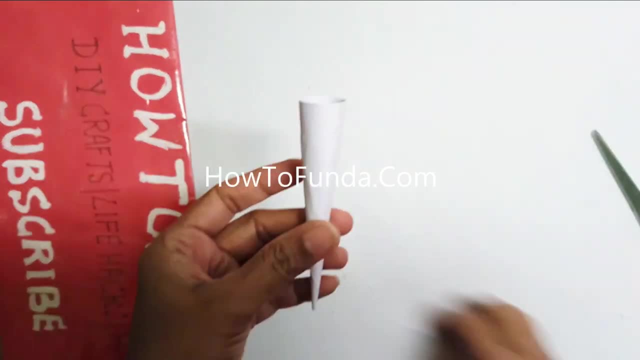 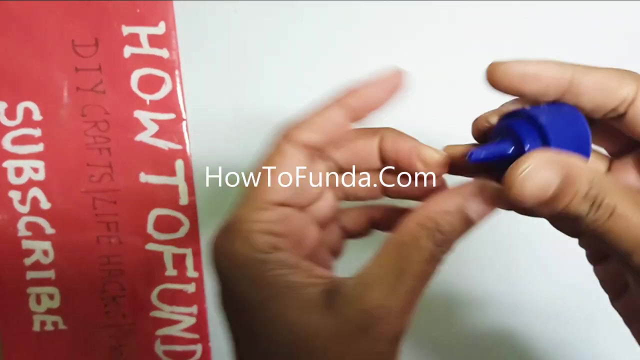 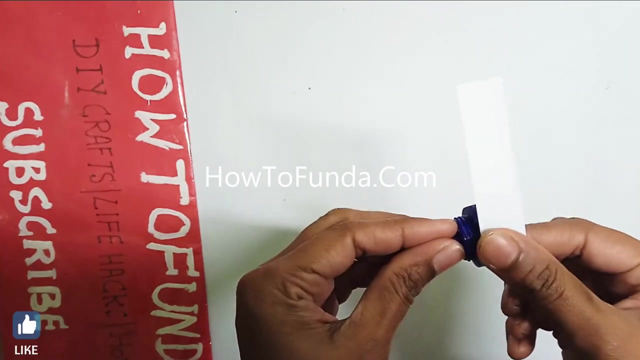 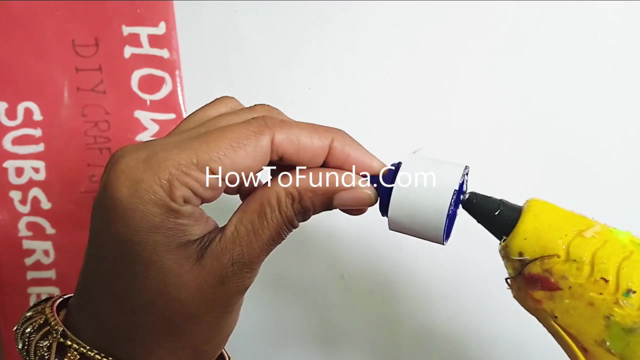 then it's your chance to be ruthless. That it's your chance to be ruthless. That it's your chance to be ruthless. They don't want to see me naked. They don't want to see me care Anytime I make some progress. 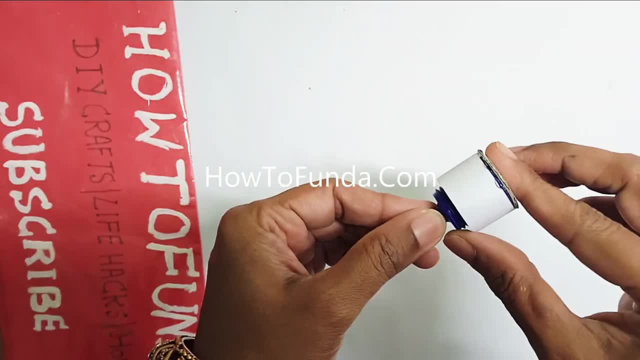 I can see that they compare. I think everyone's a little bit different. I think everyone's a little bit different. It's against me, maybe something in the air. Am I paranoid? I swear a void is forming and they're scared. 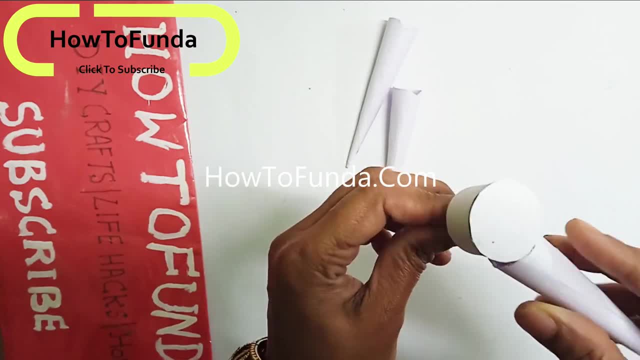 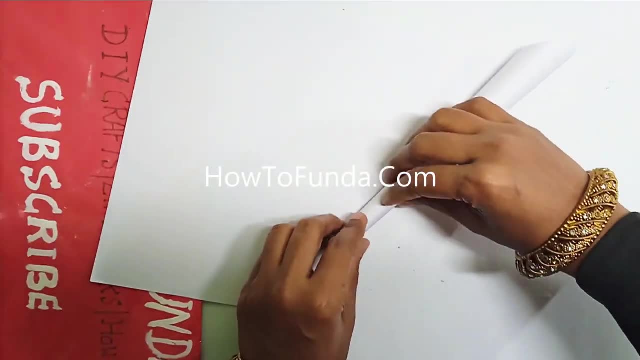 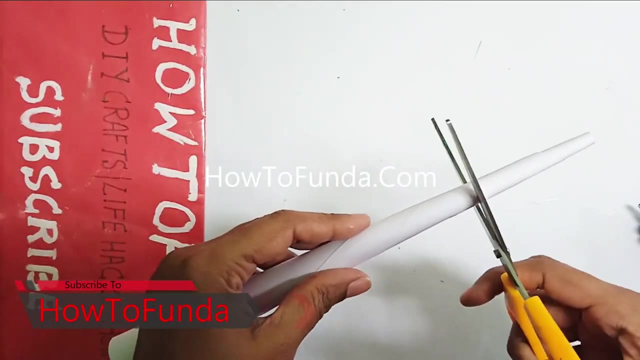 I walk a straight path. Not many can say that I like to play fast. Cross me and there's payback. You better pray that I don't see your face at any place that I go. I know you hate that. I've been doing fine. I'm not wasting any more time. I live for the fight and the climb. 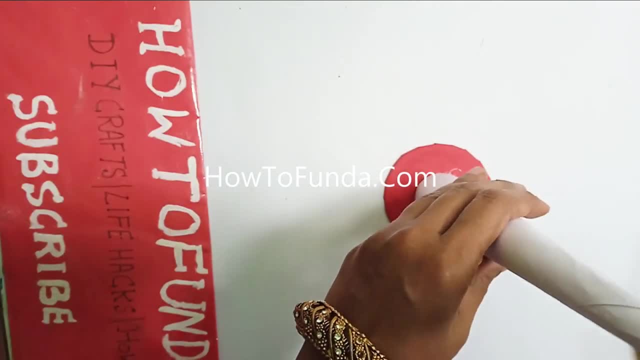 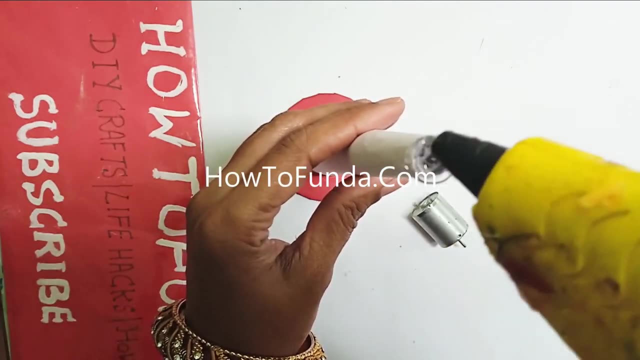 And I think that the pain that's deep inside is what divides. So I won't give up. I'm gon' make it to the top, I don't care what's in my way. I swear I'm never gonna stop. I could fall flat on my face and I swear I won't give back up. 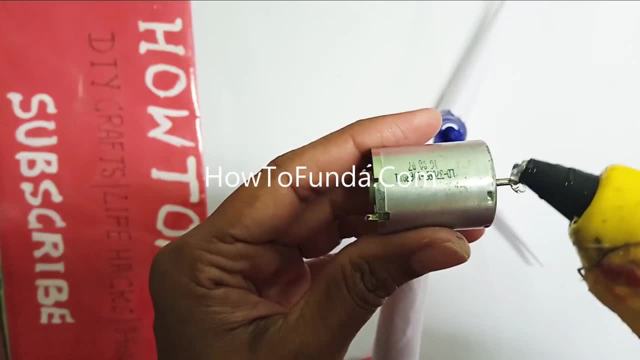 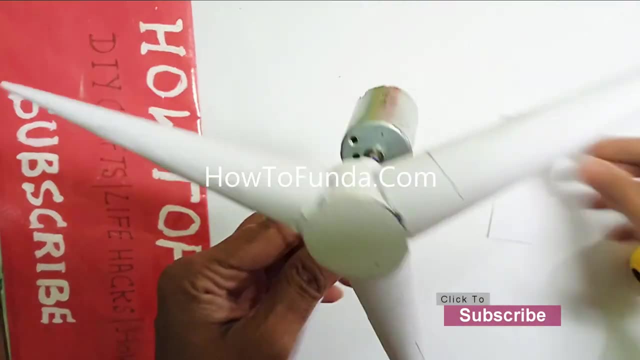 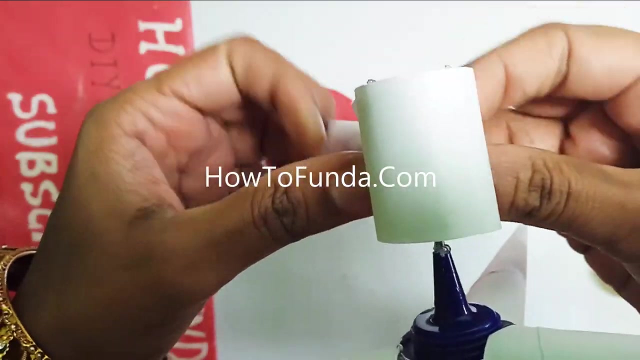 Cause I don't deserve a thing and the road ahead is tough. They'll try to kick you while you're down. They wanna rise up while you drown. They wanna fill your head with doubt. They're silently scared that you'll figure it out. I'll make it look like I'm losing. 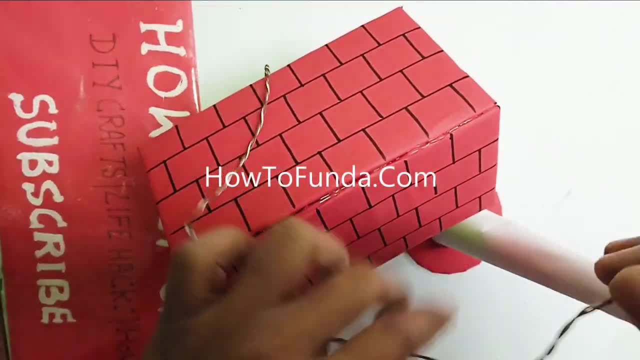 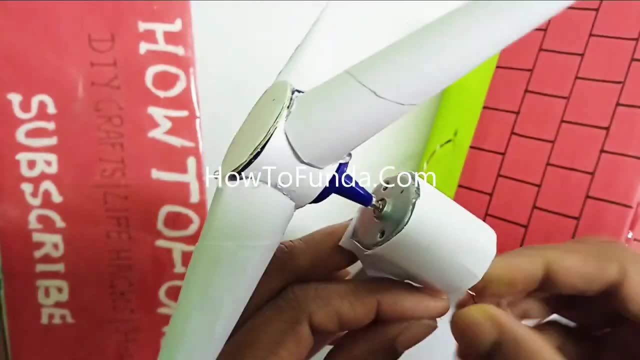 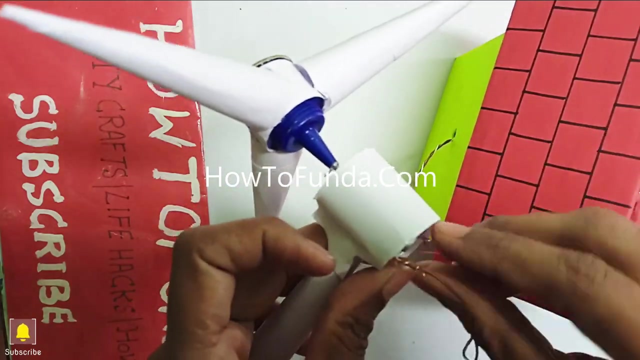 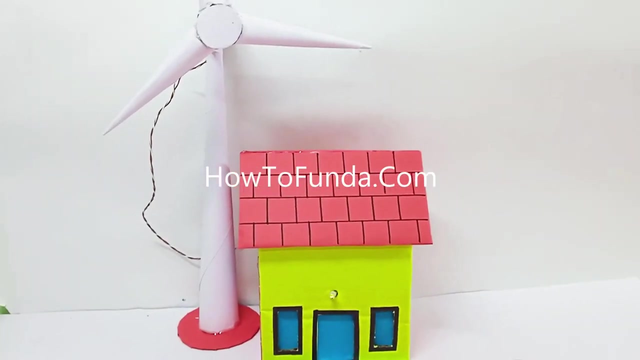 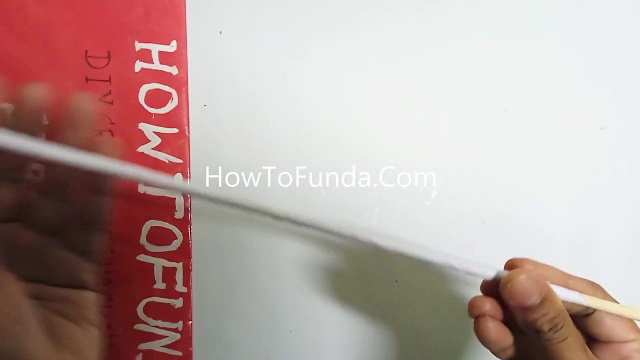 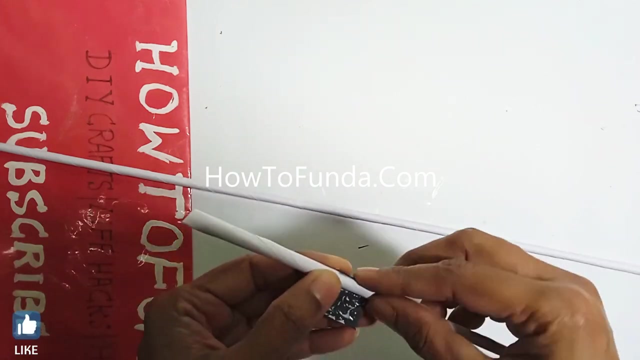